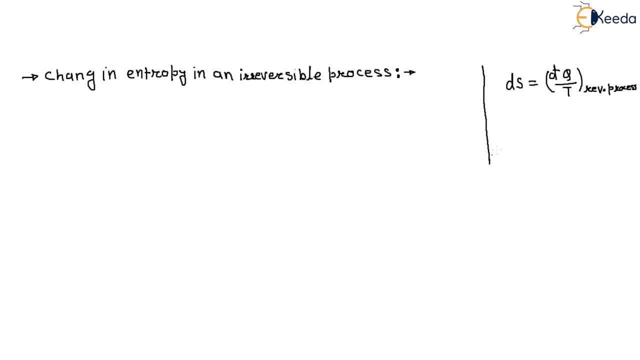 right, okay, and if you put cyclic integration to this, cyclic integration of ds is equal to cyclic integration of dq by T for reversible. this is a property. this is a property, so it is what? zero? so what is that? cyclic integration of dq by T is equal to zero. 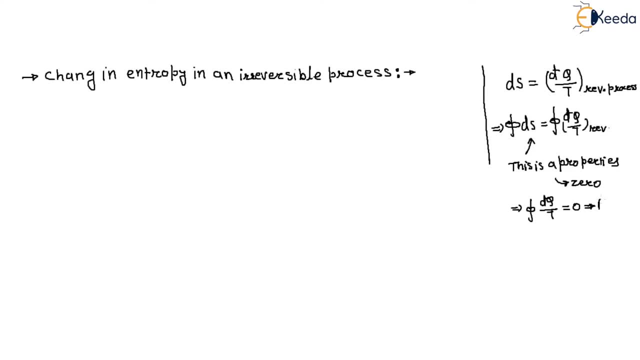 for what? reversible process? okay, now, what is for irreversible process? what is for irreversible process? so, if you take this is our cycle, if you take this is our cycle, like this one, if this is your cycle, we take a. like this one, if this is your cycle, we take a. 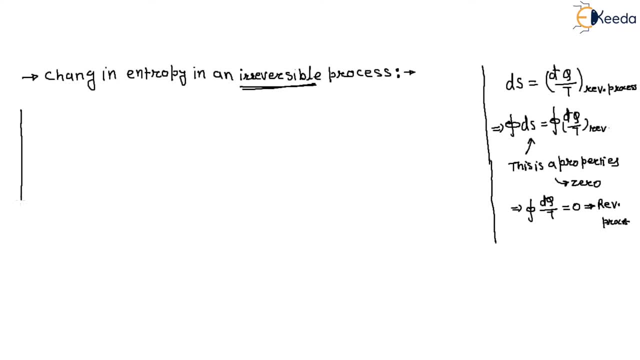 plane. is any plane which is Y and X if we take two cycle side. there is a one plane. is any plane which is Y and X if we take two cycle side. there is a one plane. is any plane which is Y and X if we take two cycle side. there is a one point and this is a two point to draw a one. 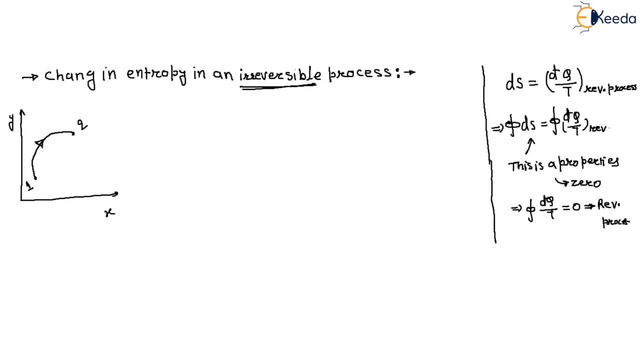 point and this is a two point. to draw a one point and this is a two point. to draw a one cycle here: one, two, two. there is other cycle here: one, two, two. there is other cycle here: one, two, two. there is other cycle, two to one. and we also join another. 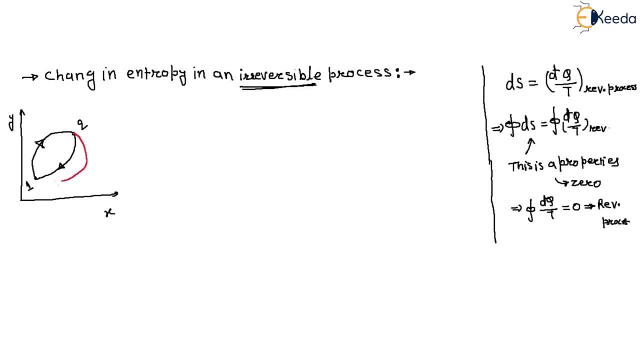 cycle two to one and we also join another cycle. so this is your reversible process. so this is your reversible process. reversible A, reversible B, and this is irreversible process. so this is your irreversible process. C- so this is C irreversible process. we take a dotted line. this is irreversible. 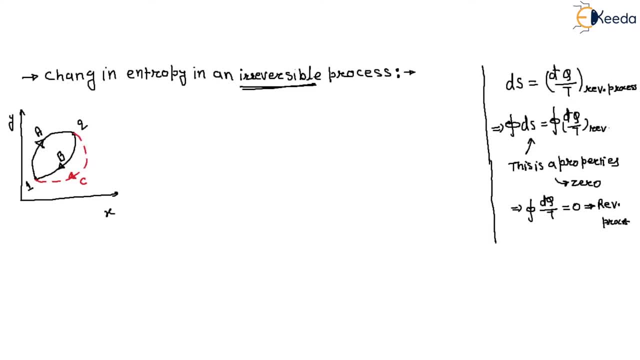 process, right, okay, so there is a, 1, a, 2, b, c. there is a, one cycle which is reversible cycle. why? because all the process is irreversible, so it's constitute a reversible cycle, but 1, a, 2, c, 1- this irreversible cycle. why? because there is any cycle in which only one process is irreversible, so the 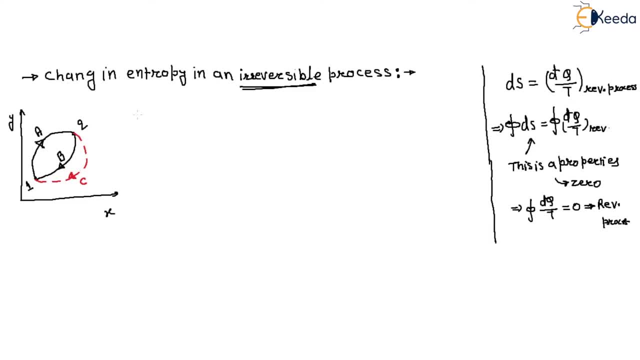 cycle is irreversible cycle. so we know that right. so what is that? if you think about what is the entropy for irreversible process? so we know that for a reversible cycle. so for a reversible cycle, for reversible cycle, what is that? 1 a, 2, b, 1- this is a reversible cycle. so for a reversible cycle, what is that? 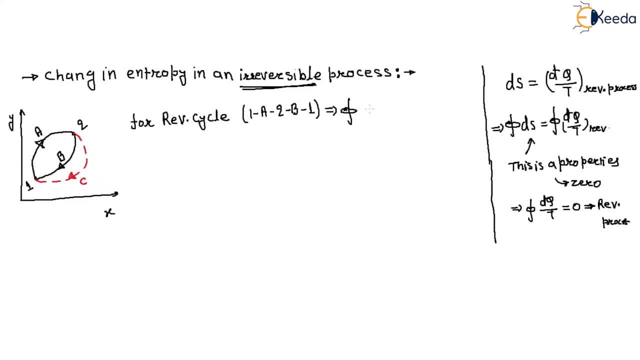 cyclic integration of dq by T is equal to 0, right. so if we take this, this is a process: 1, 2 by a path a to T via path a, plus 2 to 1 via path B. so this is your nothing: two or one to 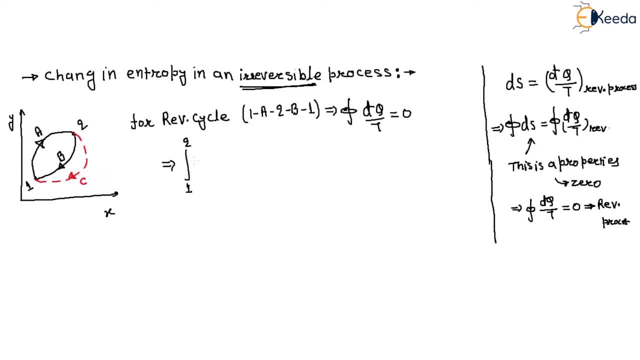 two via path a- dq by dt, plus 2 to 1 via path B- dq by T. this is equal to zerozus. you, you, you, you, you, zero, zero, two, two, right, no problem, this is your question number first. now for now, for irreversible cycle. what is that? 1, a, 2, c, 1. this is your irreversible cycle. so what? 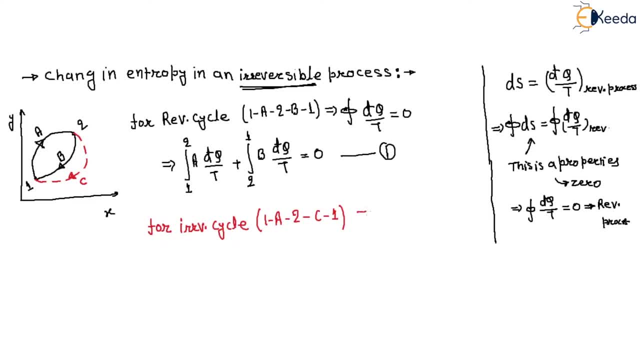 is that? so what is the irreversible cycle? so, in this case, what is the irreversible cycle? the reversal cycle is for irreversible cycle. the cyclic integration of the cyclic integral of dq by T is what it's: a less than 0 from Clausius inequality. this is from Clausius equality right. less than 0. so 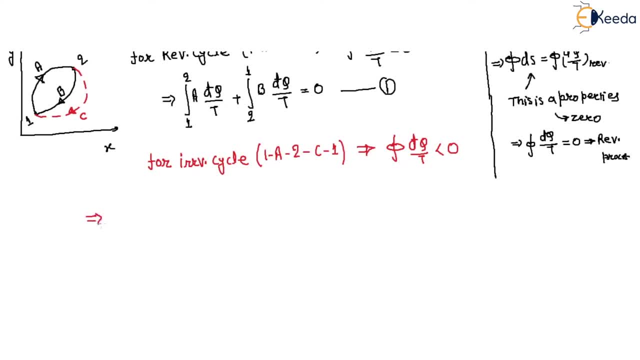 what if you take this is 1 to 2 by a path a, dq by T plus 2 to 1 by a path C, dq by T is equal to what less than 0? right now, if you put the value is: if you substitute this: 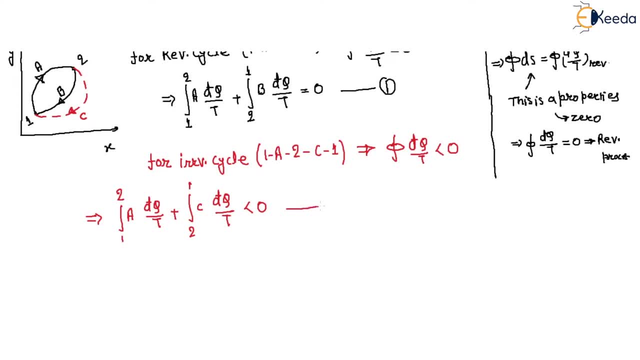 value from equation. equation: this is equation number second. what is the from first from equation first from equation first? what is that? what is that? cycling is a 1 to 2 by a path a. dq by T is equal to minus 2 to 1 by a path B. 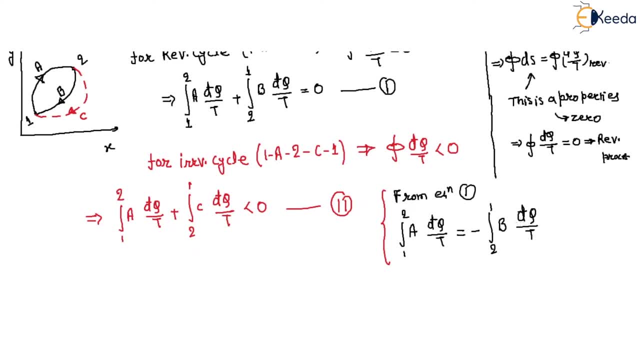 path a dq by T is equal to minus 2 to 1. by a path B dq by T. right, okay. so if you put this is negative, that means put here this: dq by T, right okay. so if you put this is negative, that means put here this: 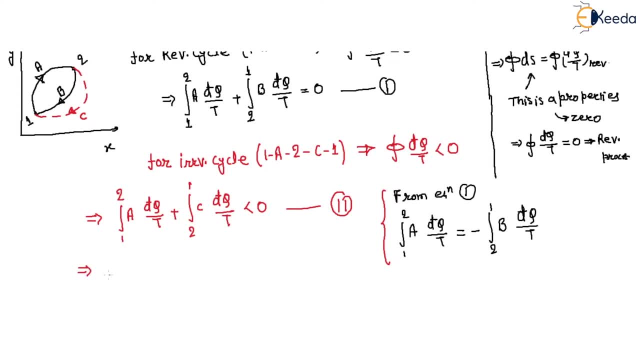 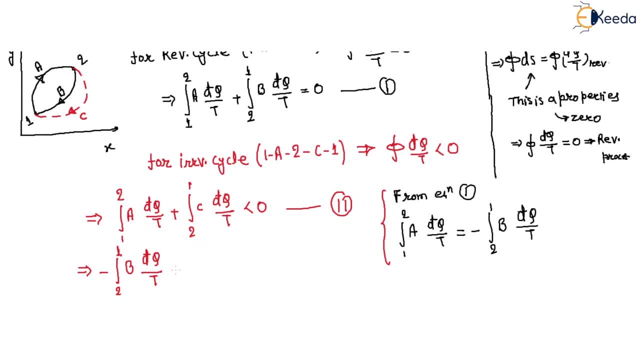 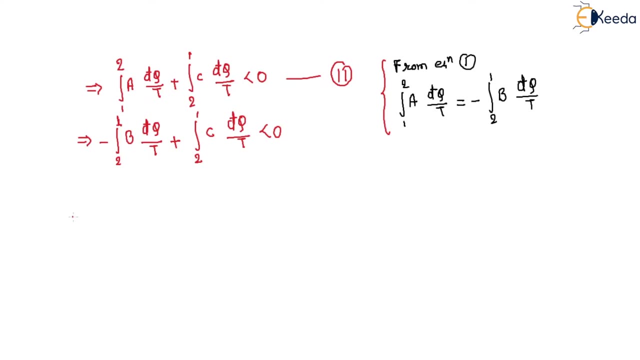 equation put here that means minus 2 to 1 by a path B, dq by T. from this equation, 1 to 2 dq by T plus 2 to 1 by a path C, dq by T is less than 0. no problem, right? so what is that? 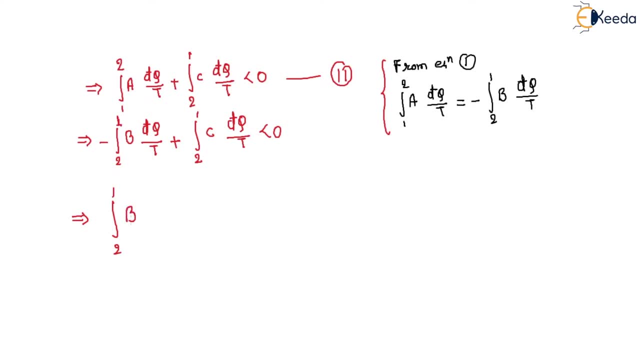 2 to 1 by a path B, dq by T is less than 2 to 1 by a path C, dq by T right. so what is that? this is for which path right? this is for for which path? this is for by a path B, and by a path B is the reversible path. so this is your. 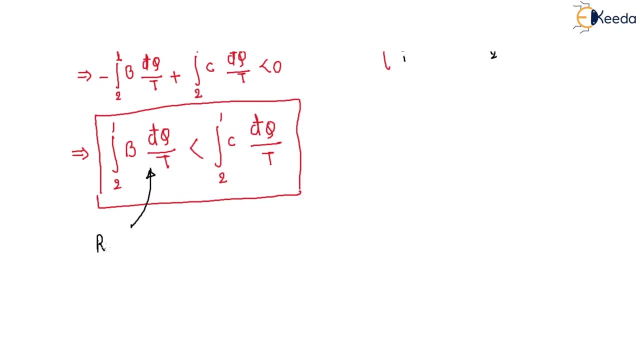 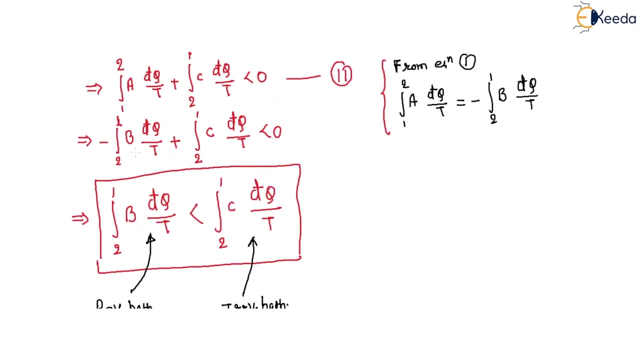 reversible path and this is your irreversible path. right, so this is irreversible path. right, so what? this is the irreversible path, this is your reversible path. okay, if you put in this side: so this is your, this is your, less than so, this is in quality, is wrong, which is actually greater than sorry, I'm sorry, this is. 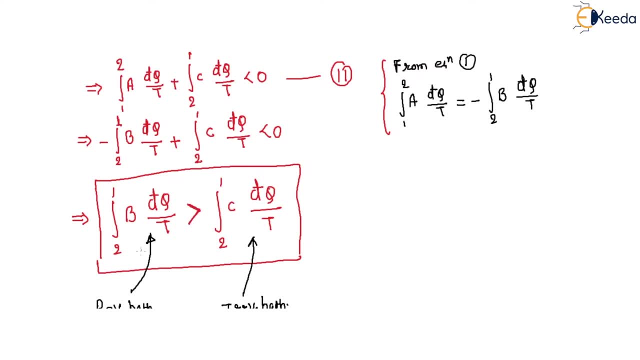 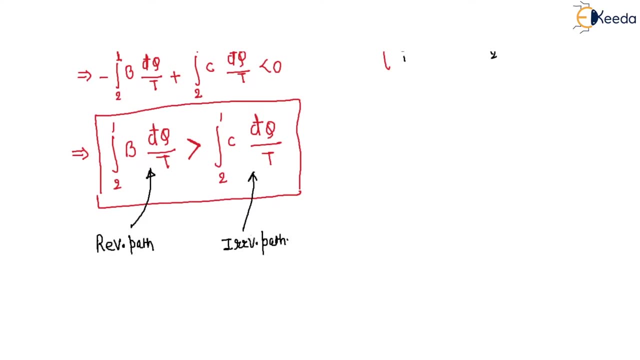 actually greater. okay, so for a reversible path, dq by T is less than 0, Q by T is higher than the irreversible path, right? so this reversible path d? Q by T is what one deltas? this is what deltas is defined, integral deltas. so what is that? from this equation you can write that delta s is greater than. 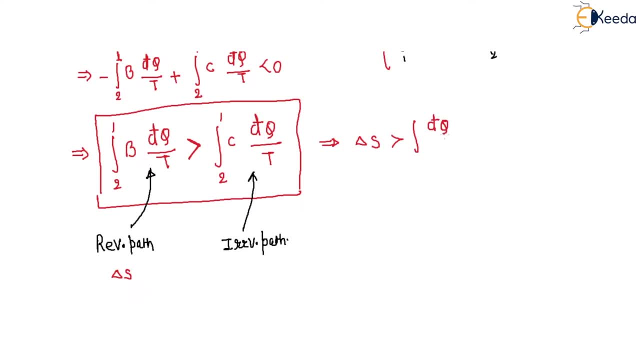 regression d, Q by T. right like that, no problem. this is for this is for irreversible process. irreversible process why? because cycle is irreversible. now, if this is irreversible, if this is irreversible, if this is irreversible, okay, so this is delta s. so if we write, delta s is equal to regression d, Q by T, for 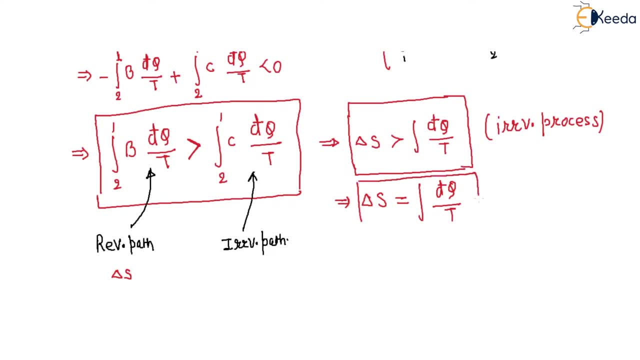 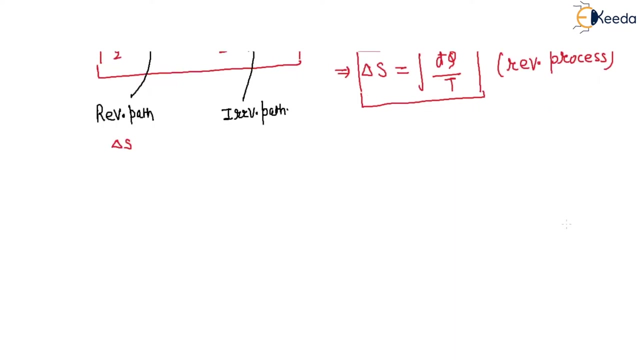 what for what? for reversible process, reversible process, no problem. right now, see, there are two equation. so if you take adiabatic process, they take process right. and adiabatic process is two type. one is reversible, other is irreversible, is irreversible for reversible. so what is your change in entropy for reversible? what is your? 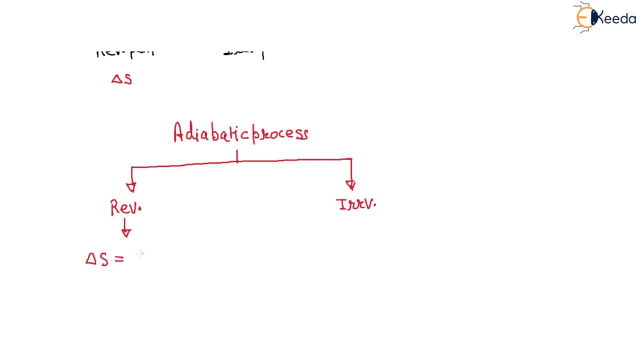 change. entropy delta s is equal to integration d, Q by T and for irreversible. what is the change? in entropy delta s is greater than dq by T, right, but for adiabatic. but for adiabatic adiabatic dq is equal to 0, so this is 0 and this is also 0. so reversible adiabatic. 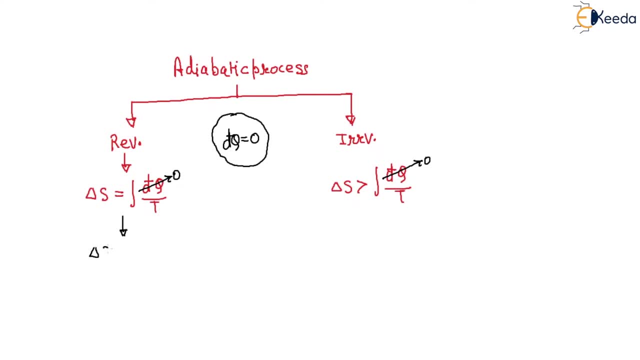 process is what delta. s is equal to 0, that means s1 is equal to s2 is equal to constant. so entropy is constant, so it is called. so it is called isentropic process, right, isentropic process, no problem now, so this is what delta s. 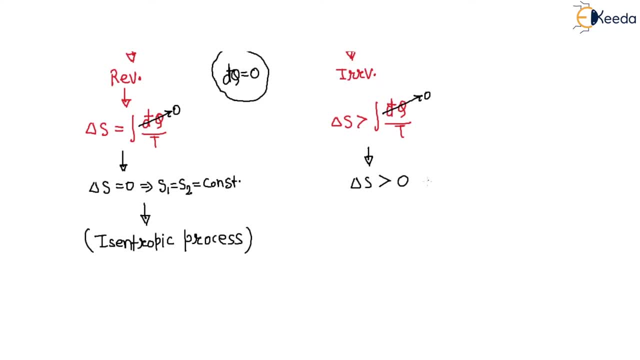 always greater than 0, if delta s always greater than 0, so s2 minus s1 is greater than 0. so what is that? s2 must be increased. so entropy will increase. so in this case, what is that? entropy must be increased, must be increase. so what is that? so if adiabatic, reversible and adiabatic process, 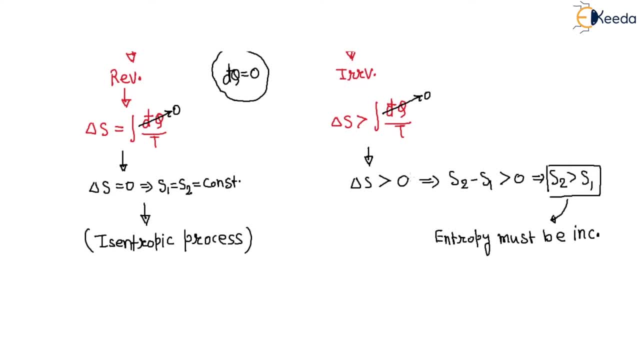 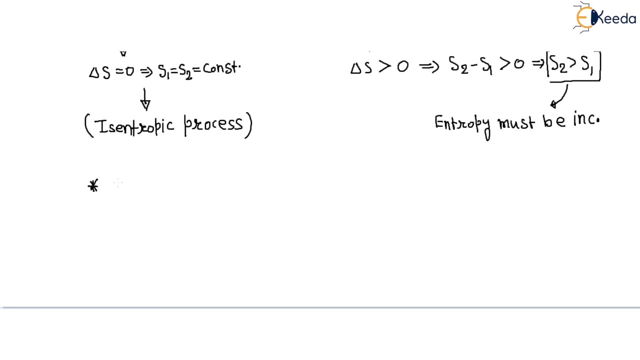 isentropic process and irreversible and adiabatic process. entropy must be increase. okay, no problem. so what is your conclusion? the conclusion number first: reversible plus adiabatic process. what is that entropy? reversible plus adiabatic process. isentropic tropic process. 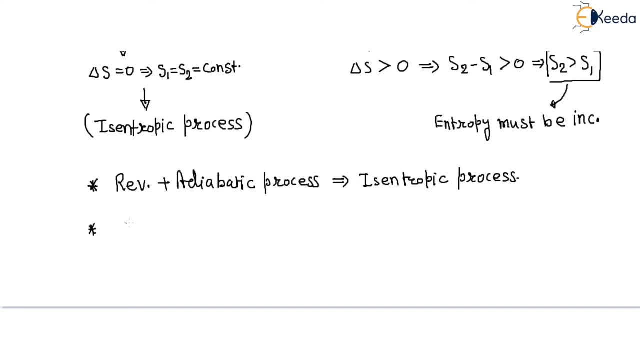 number. second use to substitute all two: irreversible plus adiabatic process. What is that? Entropy must be engaged, So it is not necessary that adiabatic process is isentropic process. No, it is very wrong. So keep in mind What is that Adiabatic process? 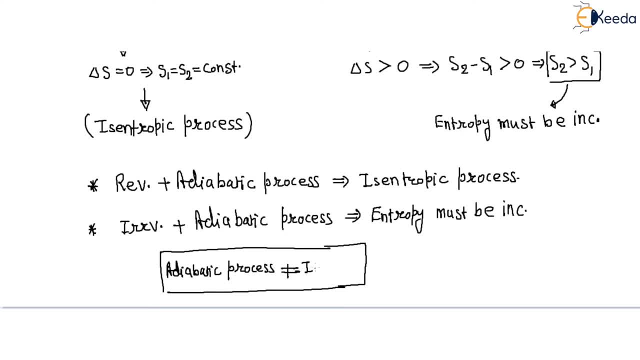 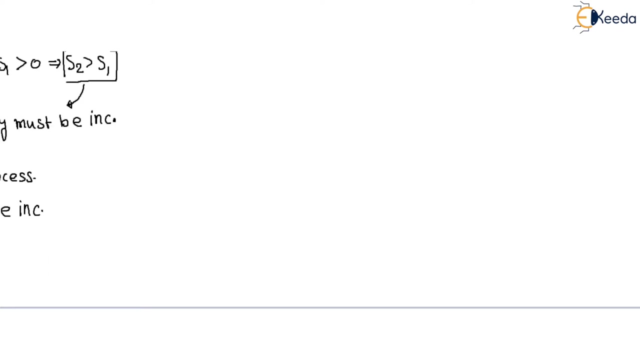 That means it is not isentropic process, Right, Okay. Another thing is that: what is that Here, if you see like that? So what is that You see like that? Okay, Now, what is that? So for irreversible process? 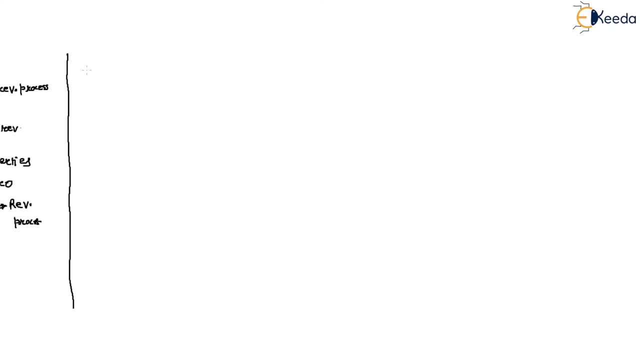 Okay, So for irreversible process. what is that? So we can write that for any process. So for any process. what is that? Delta S is greater than equal to dq by t. Yeah, q by t. Anything is nothing Integrated. 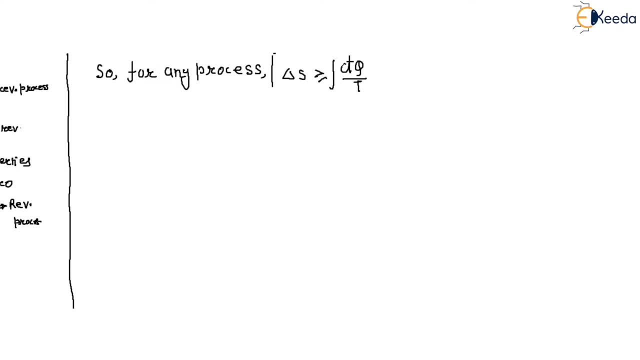 Integration, Integration dq by t. This is for any process. No problem, Right, Okay, Now for irreversible process. What is Delta? S is greater than integration dq by t. No problem, There is no problem, Okay, There is no problem. That means what you can write. that, That means you can also write: 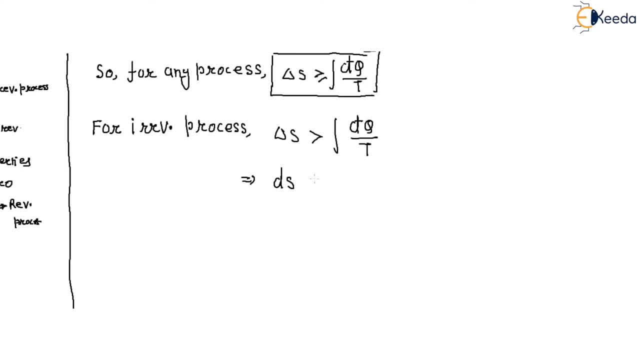 that ds is greater than dq by t. There is no, any problem, Anything, No problem, Right? So from this you can see that Okay, Okay, Okay, Okay, Okay, Okay. Then, if you look frozen, You can write down dq by t, c plus dq by t. 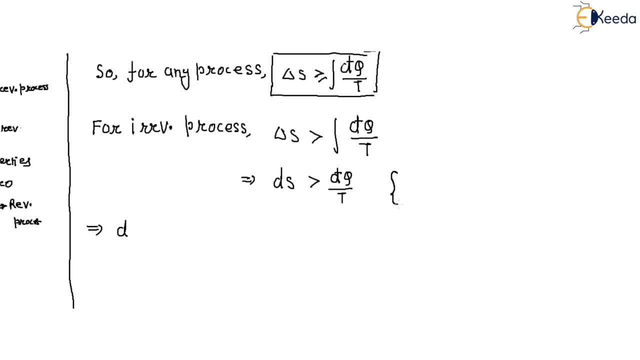 dq by t is equal to d and then dq by t is equal to d, q by t. If we change the inequality with equality, if you change with inequality, that means, if you think about that, there is n value. M is greater than N. So if you change the inequality, M is equal N. you must be at some positive quantity. 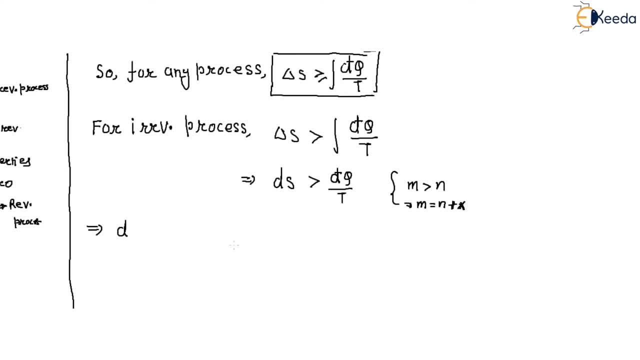 You must be at some positive quantity, No problem, You must be at some positive quantity, Anyway, all that is right. Yeah, leave it for the course. only the whole thing. positive quantity if it is 0, that it is exactly M equal to n and it is greater. 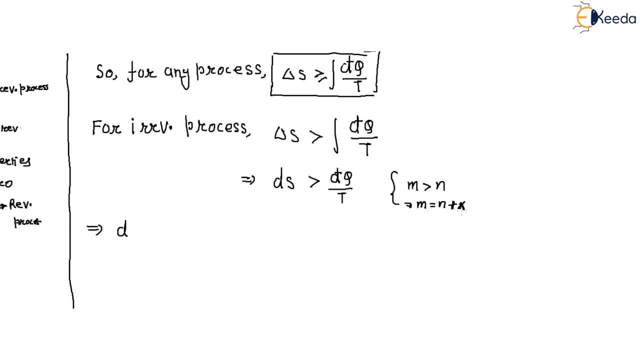 than 0, that means this will greater than 0. so right, so it is positive quantity. so for this, M is greater than n. M is greater than n. for which process? for irreversible process. so if you add X and X have some value other than 0. so this: 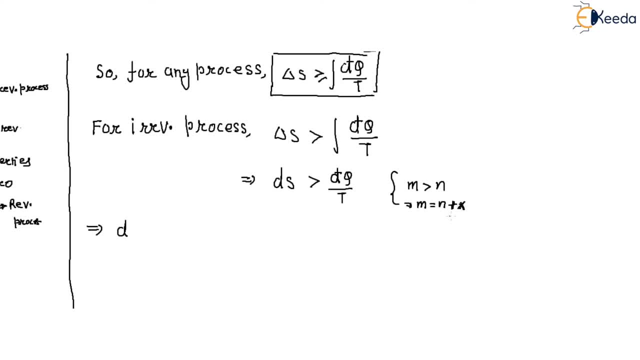 is for irreversible process, so this is for irreversible process, and if X equal to 0, this is for reversible process. see this is for what process this is. M is greater than n. for what process? for irreversible process? irreversible process. so M equal to n plus X. for which process? irreversible process? why we got this and 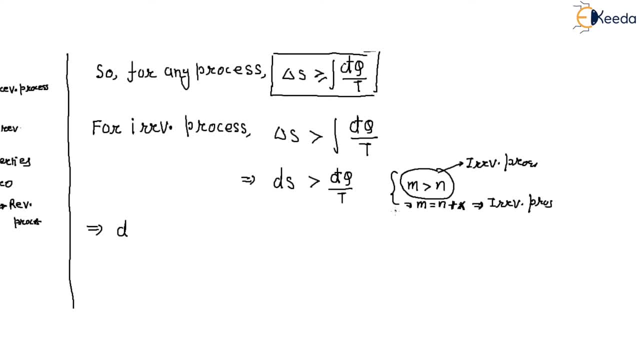 this equation are same. now. if so, for irreversible process, if you add something, so this x is positive or negative. this is positive value, right? if x is 0, so n, exactly n, or n is what ds, n is what dq by t, so ds is equal to dq by 2. when, when the process is reversible, you think like that here. 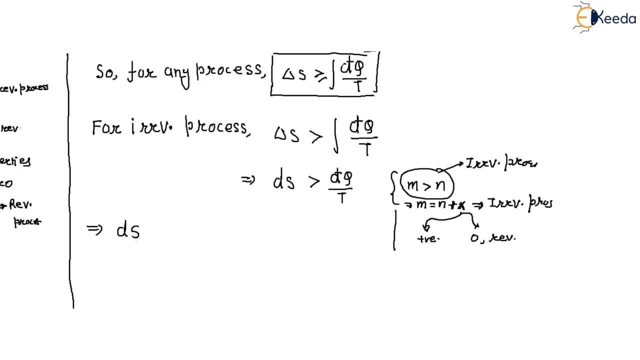 right. so this ds, so this ds is what. this ds is equal to dq by t plus you add some positive quantity x, x, some positive quantity x. so what is the range of x? what is the range of x if x greater than 0 for irreversible process? 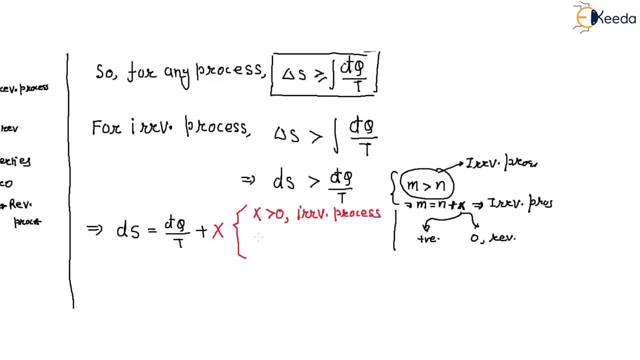 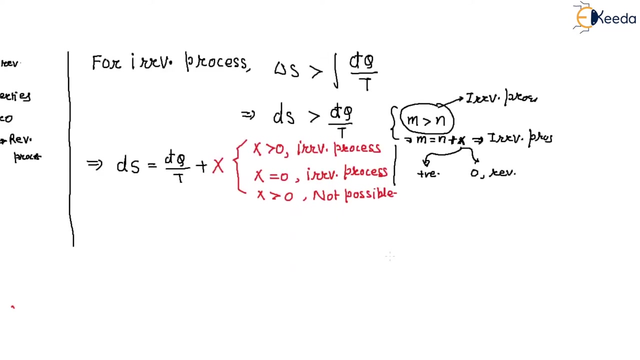 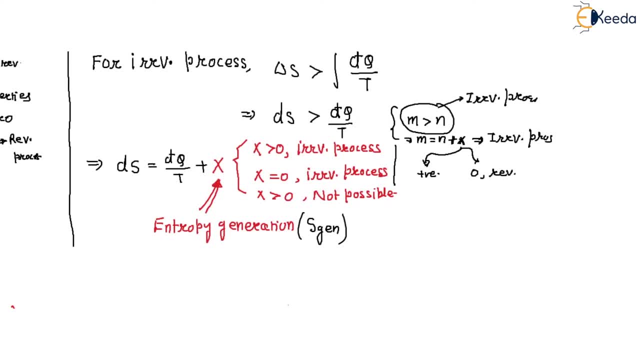 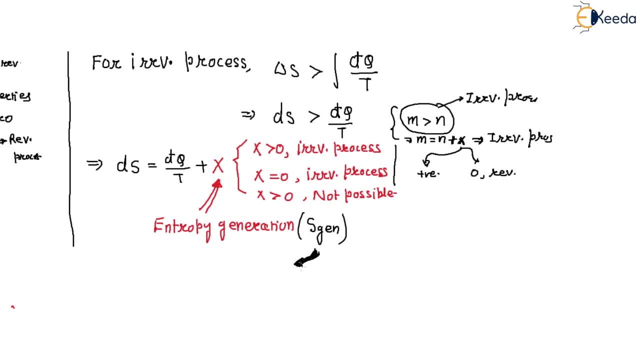 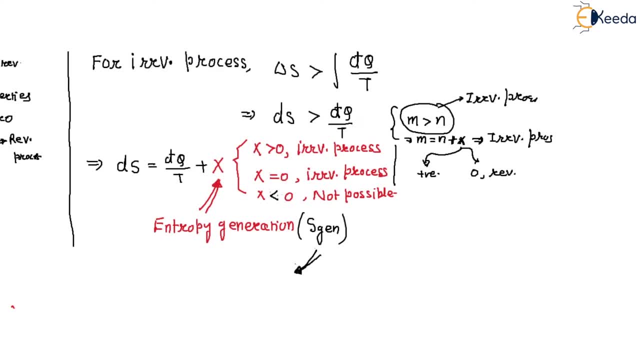 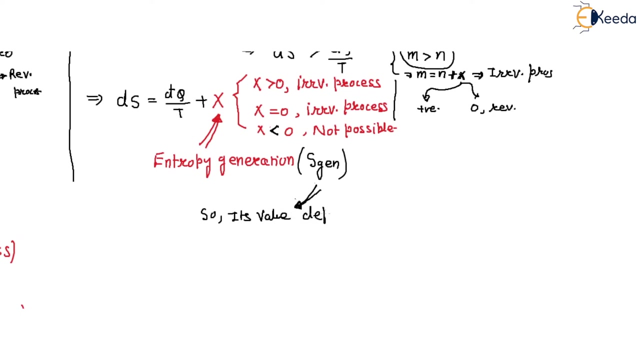 greater than x, less than x, not possible. okay, so entropy generation is what it is: a value that means. if x generation greater than zero, irreversible process. generation less than zero, equal to zero, irreversible process, so this is your for process right. so its value depends upon the process. so its value depends upon the process. 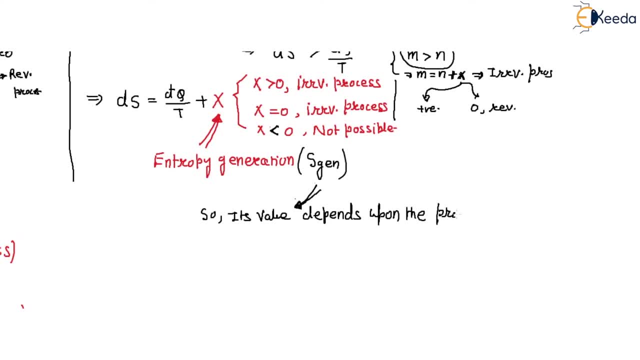 which process to be followed, process to be followed, right, this is your for process. so it is a, not a property. if this is a process, if this is so, this is depends upon path. this is for process, those. so this depends upon path, so path of the process. 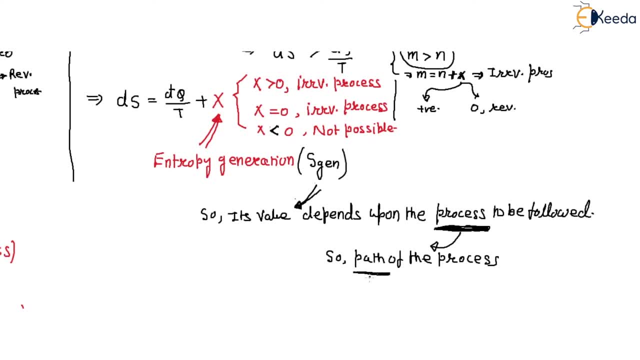 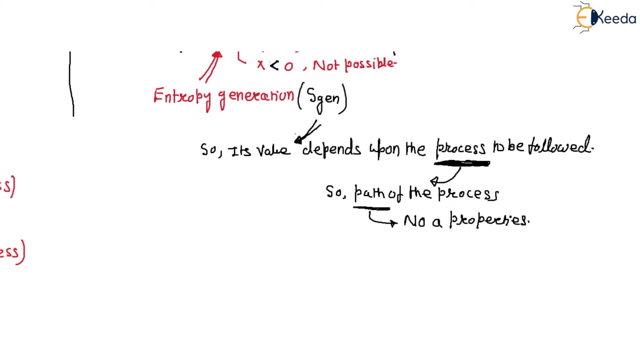 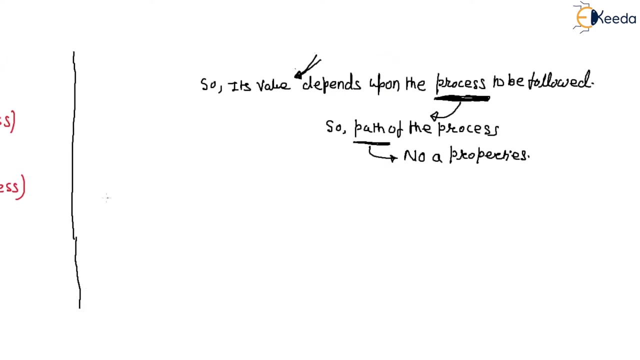 if it depends upon the path. so it is a, not a property, not a right, it is not a property. okay now. so one note point here: is that very important, very important? i'm telling you see, what is that? entropy generation? entropy generation, that means s, g, c, n. 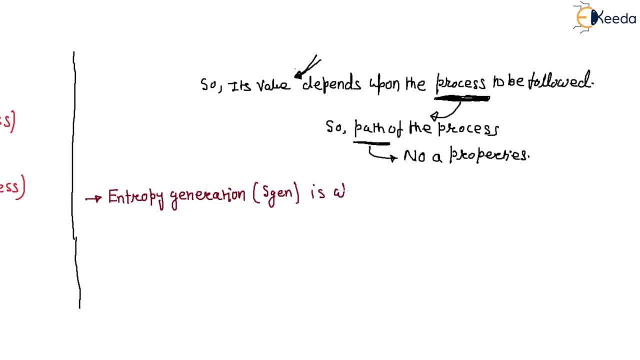 c, n is always, is always a positive quantity. quantity or zero, right or zero, its value depends on the process, on the process, and thus it is not a property, not a properties of the system. right also, in the absence of any entropy transfer, the entropy change of a system, 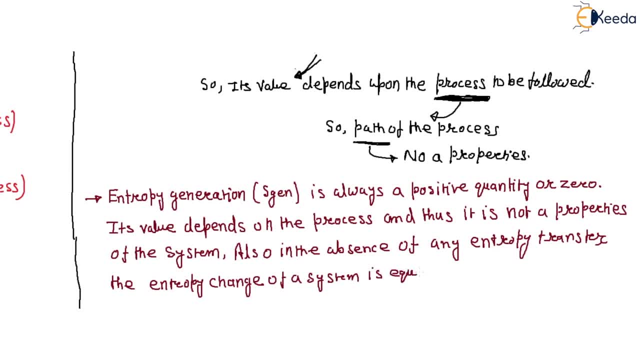 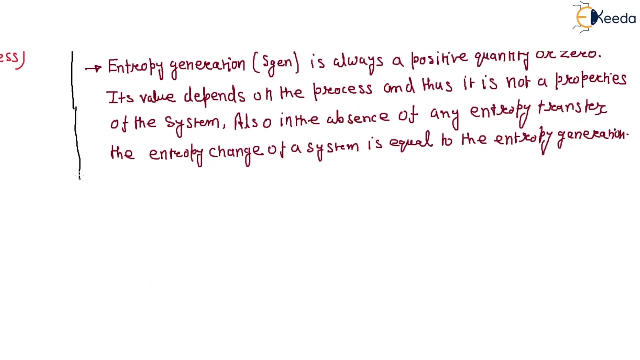 is equal to the entropy generation, entropy population. see this equation. what is say that? ok, this is like that. if that means, what is the equation? delta s of the system is equal to. this is for: system is equal to s2 minus s1 is equal to integration 1 to 2. 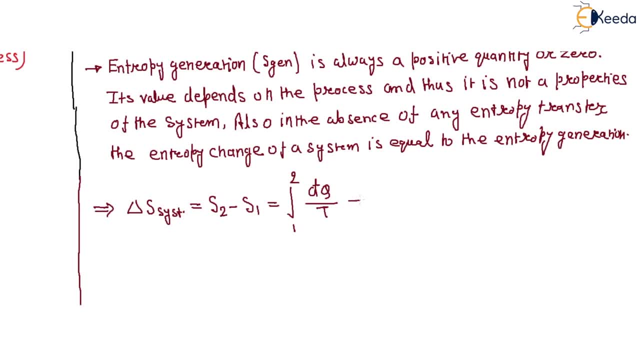 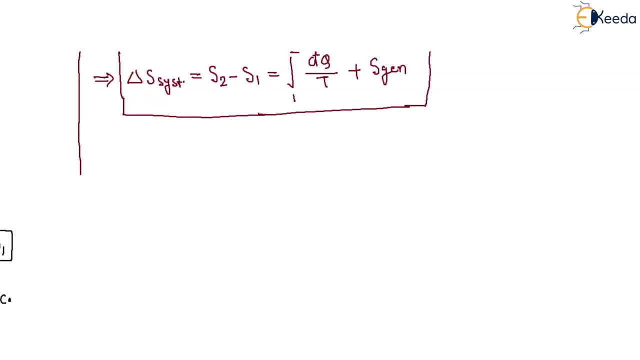 dq by t plus entropy generation. this is your equation. this is your equation, right. so see, very clear to you and I am very clear to you right. how see this s2 minus s1, this s2 minus s1 is what? what is s2 minus s1? 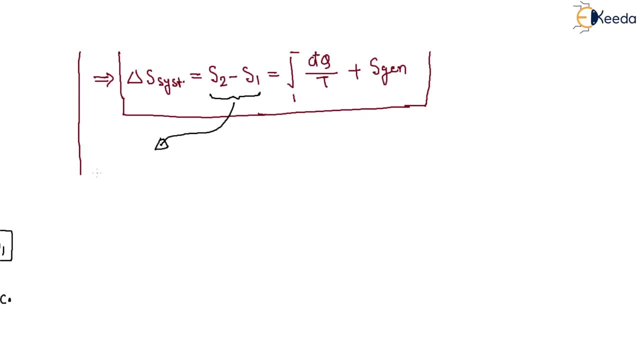 what is s2 minus s1? entropy: change of the system, the change of the system right. what is this one? what is this one? this is your. entropy transfer due to heat right. and what is this one? what is this one? what is this one? this is your. 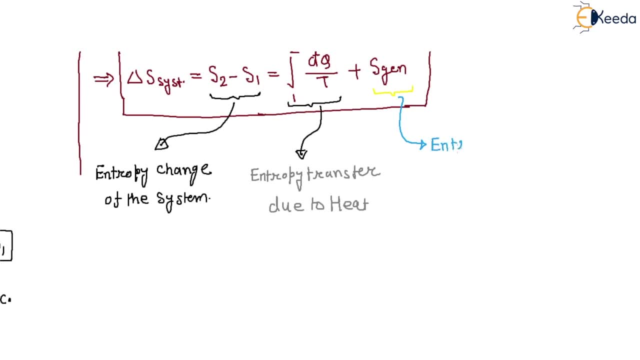 entropy generation. entropy generation, that means, what is this one? what is this physical meaning? this measures the extent of irreversibility physically, physically. this measured, this measured of the extent of irreversibility, this measure the extent of irreversibility. that means higher is the higher entropy generation. 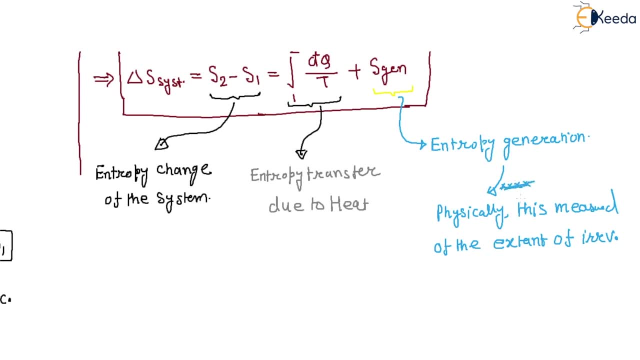 higher is the higher irreversibility, lower is the lower entropy generation, lower is the lower irreversibility. and if this is zero, the irreversibility is zero. that means totally. the change of entropy of the system is equal to entropy transfer due to heat. so one point is here that 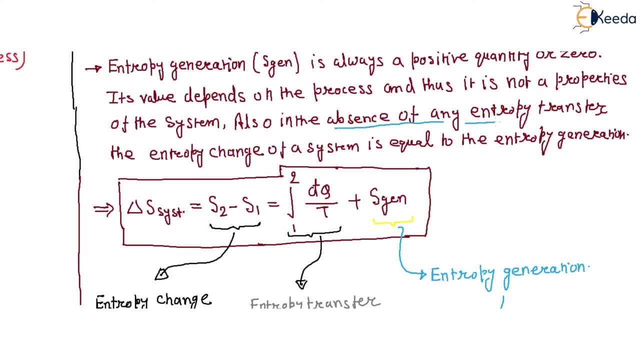 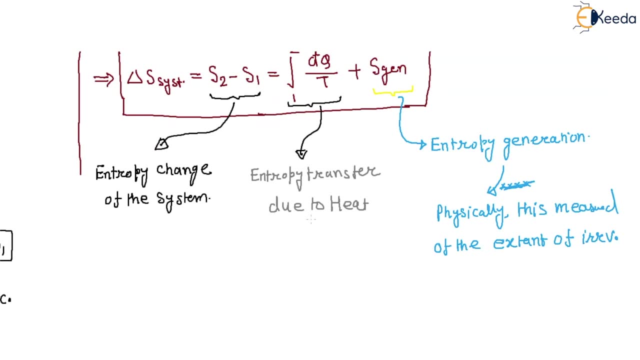 absence of any entropy transfer. that means if the entropy transfer value zero, so the entropy change of the system is equal to entropy generation. so right, if this is zero, if this is zero, when zero, when zero adiabatic. so dq is zero. so if dq is zero,